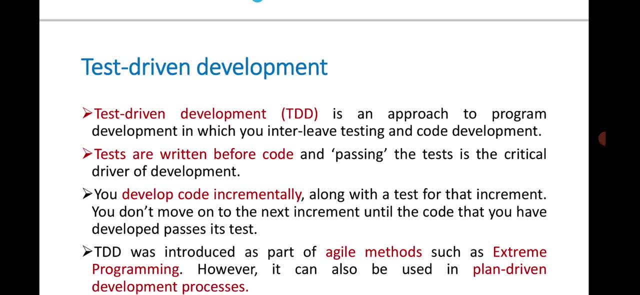 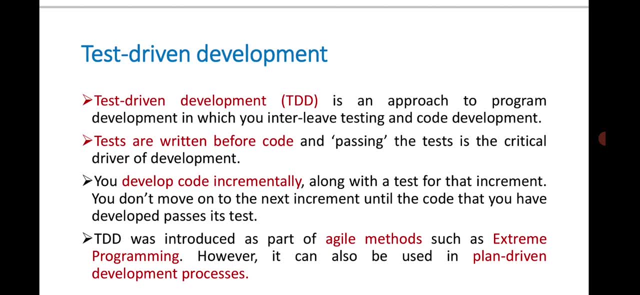 as well as code development. So both the activities will be get mixed here. Okay, So that is the specialty of test-driven development. Okay, So here the tests are written before the code, and passing the test is what The critical drive of the development. So here, 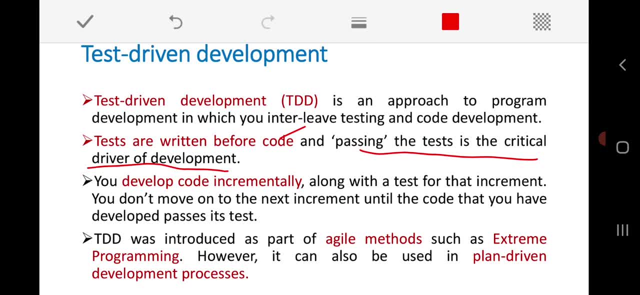 whatever the code that we are planning to write for that particular coding, before implementing that code, we will write a test for that. Okay, So we are writing a test in the sense of what, How that particular code That we are planning to write is to be get tested, with what input data that we need to. 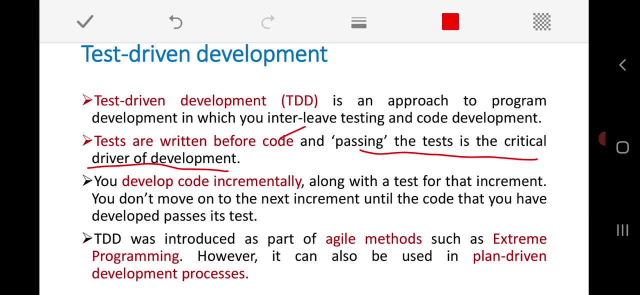 test. What is the expected output of that? Okay, So that is called as what? The test-driven development? Okay, Or even, especially in case of extreme programming, is one kind of concept, So, where we are going to use this test-first development. Okay, You can also call it as: 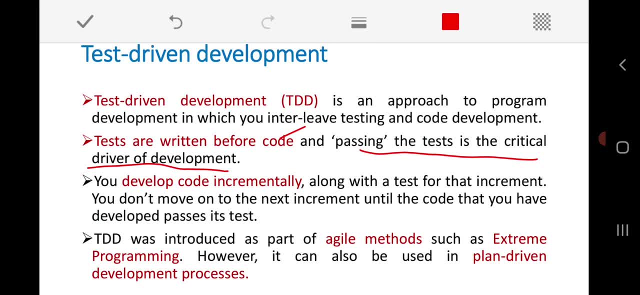 a test-first development. So means before writing the code we will be ready with what, How to test that particular code. That is the basic theme of what Test-driven development. So especially here, we are going to develop the code incrementally, Okay, And along with a test for that. increment means: 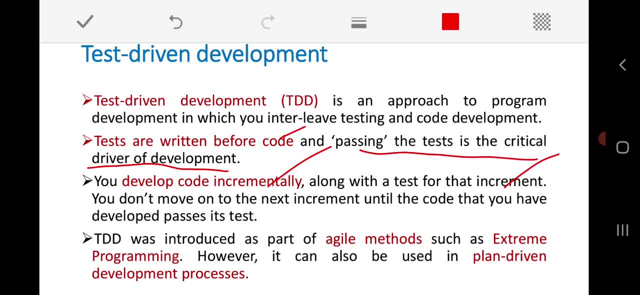 not only we are developing the code incrementally, for every increment we are going to come up with what test that increment is to be get tested. So here, we are not going to move on to the next increment until the code that we have written. 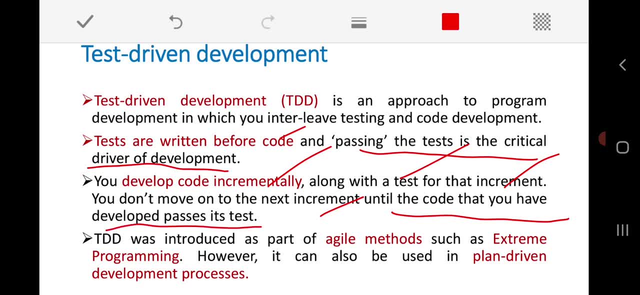 or developed passes to what that particular test see. for example, say, if i am implementing two different increments like the username and password, these are the two different increments. okay, so until and unless the code returns to check whether my username accepting- accepting of the username- is going to be get working properly or not, okay, that will be get tested. 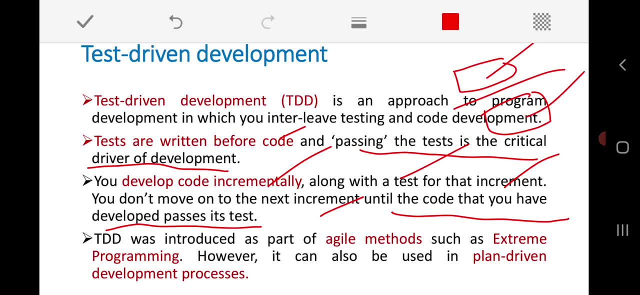 first, then only, i will go for accepting what. i will be writing a code to accept what, the particular password, and that will be get tested next. so, like this, increment by increment, we will be developing the code and before developing the, every increment, we will be ready with the test case that is test. 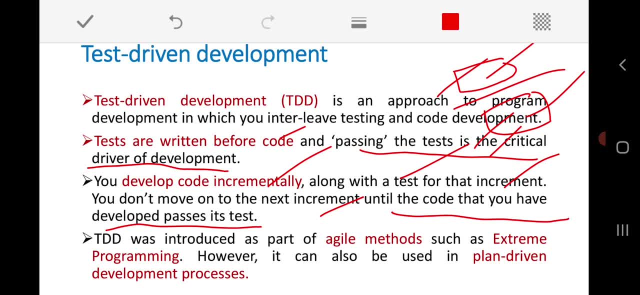 that will be get designed and it will be get tested immediately after that increment is going to be: get what get developed. okay, so this is how the test driven development is going to work out, and just now, as i told that, so this tdd was introduced as a part of agile method. 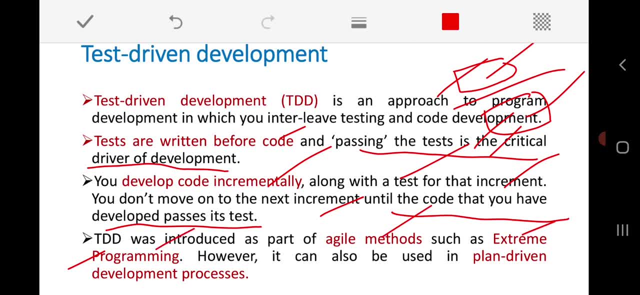 such as extreme programming- okay, even it's a very popular kind of the software development concepts, that's agile method and extreme programming, where this test driven development is very popular one, and also this tdd can also be get used in our plan driven development process also okay. 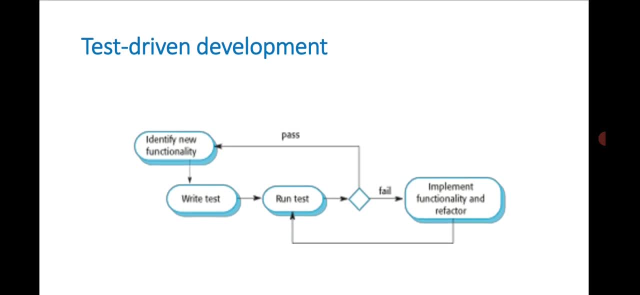 so just have a look at the very simple diagram of this test driven development. so here, every time, we will be starting with a new functionality or the particular increment of the particular functionality. then, before going to implement that functionality, first we will write what the test okay. then we will run the test. okay. when we will run the test, either it will be. 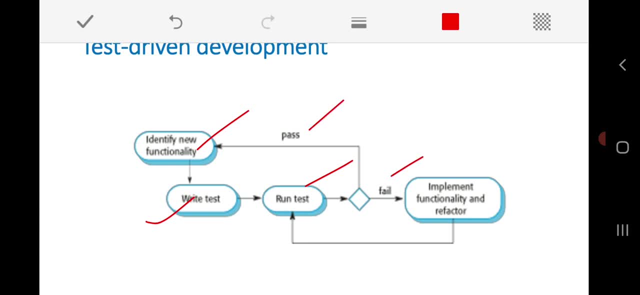 get pass or you may get fail. okay, if the test is going to be get passed, then we will run the test. okay, then only, we are going to move with what? the next increment of the particular functionality. if you are going to get fail, then automatically, once again the functionality. 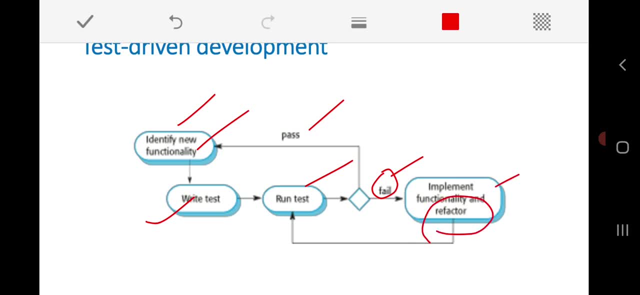 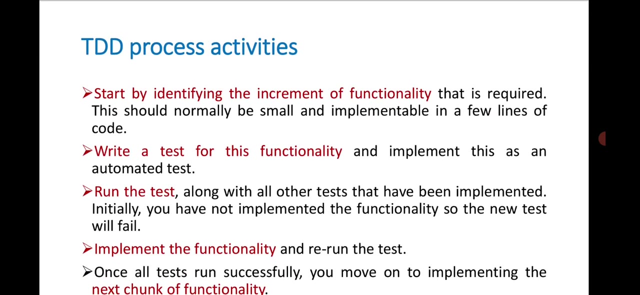 will be get implemented with what. refactoring means changing or improving the quality of the code. we will modify that functionality and it will be get what retested. so this is how the test development is going to work out here. so just have a look at the ttd process. 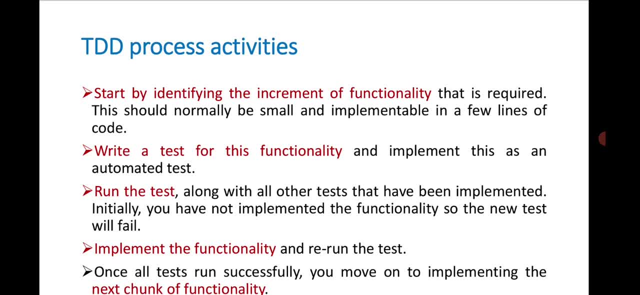 activities here. so here we will be always going to start with identifying the increment of the functionality which is required. then this should be: normally it will be a small and it should be implementable increment of that particular functionality which is having a few lines of code. okay, then we are going to write a test for this functionality and 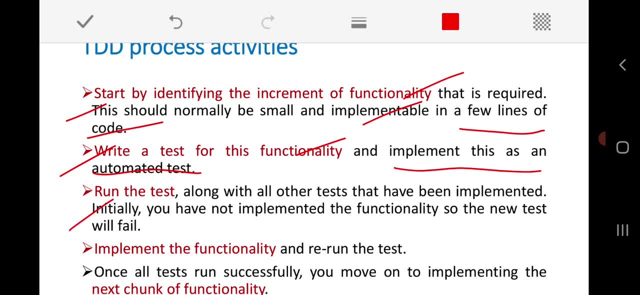 implement this as an what automated test. okay, then, initially we are going to run the test along with all other tests that have been already implemented and normally, initially, in the first attempt, normally our test is going to be get failed here. so why? because we have still not yet implemented the functionality. okay, so our very first test will be always: 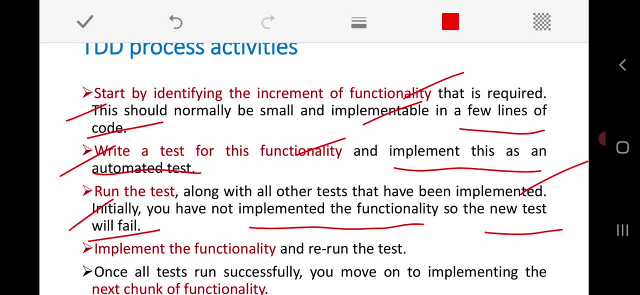 it will be get failed. but after getting failed, we will implement the functionality with proper logic and it will be get retested. okay, that is what we will. we will go forward, implement the functionality and we are going to rerun the test and finally, once all tests run successfully, 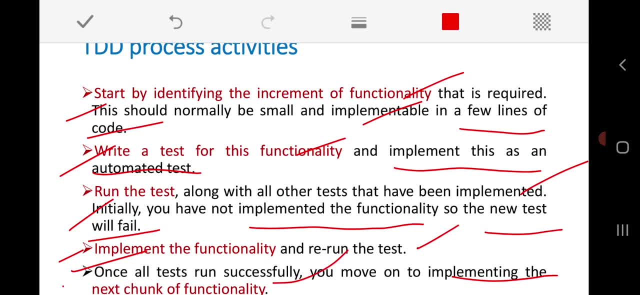 we are going to move to implement what? the next chunk of the functionality. so it means that we are implementing the functionalities increment by increment. okay, and for every increment, in the initial stage itself, the test will be get designed and every increment will be get tested with that particular test. okay. 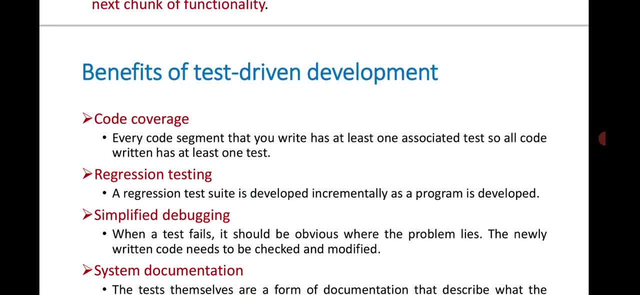 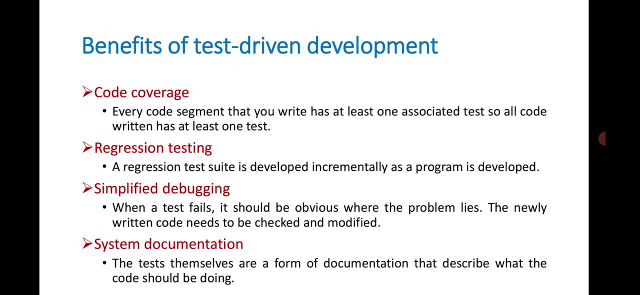 So let us have a look at the next part of the test. so what is the benefits of the test driven development here? so what are all the different benefits that we can come across with this test development is test driven development is concerned. just have a look. 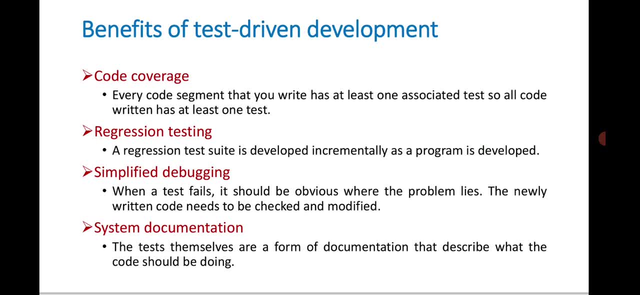 at there. the very first benefit is the code coverage here. so here, as we are going to test the code part by part or increment by increment, so here, every code segment that we are going to write, at least one test will be done on each part or each segment of the code, so that 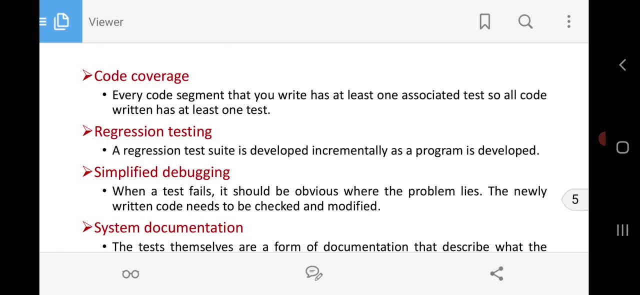 by the end of that particular implementation of the functionality is concerned, the each and every part of the code will be: get what tested, that we can call it as a code coverage here, okay, and then the regression testing. so here the regression testing in the sense, here the regression test suit is developed, what incrementally as a program is what developed. 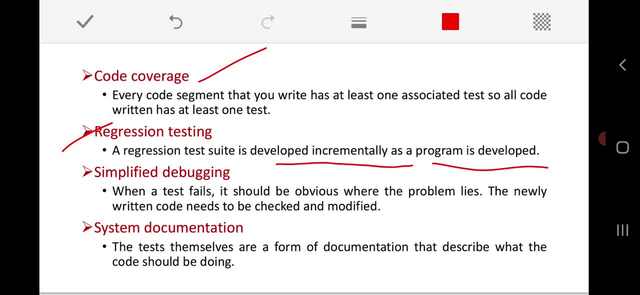 okay. so basically, if you just try to recall the concept of this test driven development here we told that we are going to test not as a functionality as a whole. here we are going to implement that functionality increment by increment and after testing the every increment of that particular functionality, it will be get combined with the next set of function. 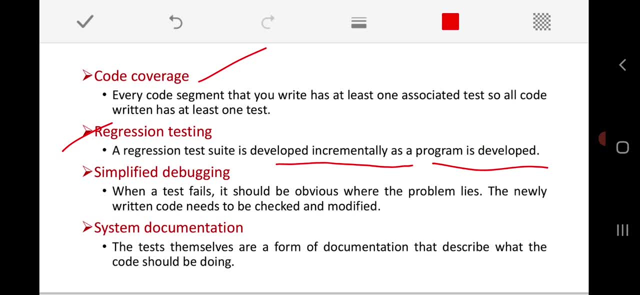 increment and while doing the testing of that particular increment number two of that functionality, once again, the test will be get repeated on both increment one and what increment two. okay, so, so that in case of regression testing is concerned, we always used to make sure that there should not be any kind of breakdown. okay, so, in case of that overall implementation, 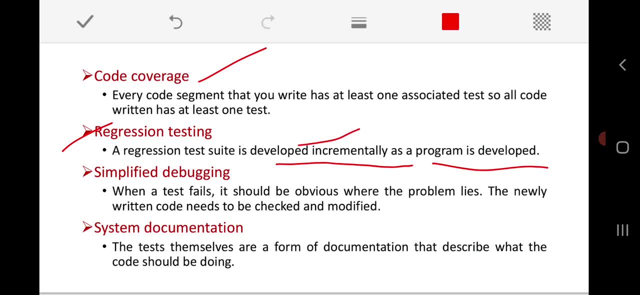 of the functionality is concerned, so that care should be always taken. and the another advantage or benefit here is simplified debugging. so here, whenever the test is going to get fail, it should be obvious where the problem lies, that we can easily identify why. because we are implementing the functionality chunk by chunk, that is, increment by increment. okay. 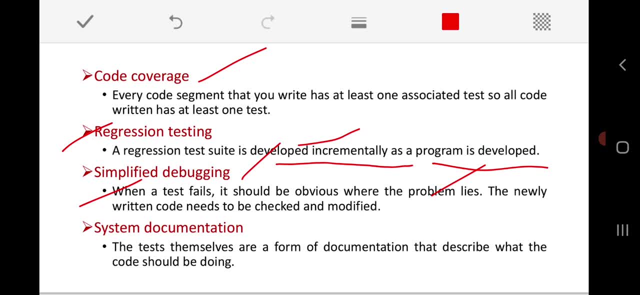 so it is guaranteed that the particular identified bug or the, whatever the failure that we are going to be doing in this particular part of the system itself that we can very easily identify so that it will be a simplified debugging and finally, the system documentation. so, whatever the series of tests that we are going to perform here, those tests themselves are going to make. 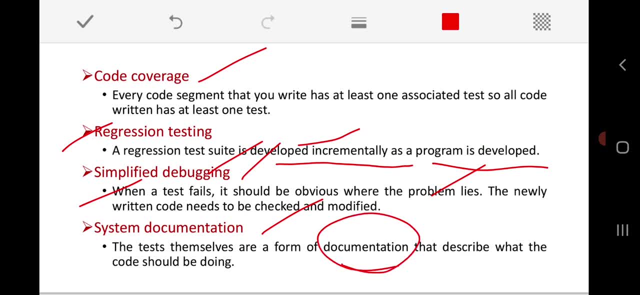 a, or they are going to create what, as if they are going to be act as a documentation here. okay, and this documentation is going to describe what the code should be, what doing, so that we can very easily understand that, what a test is, and we can easily understand that. 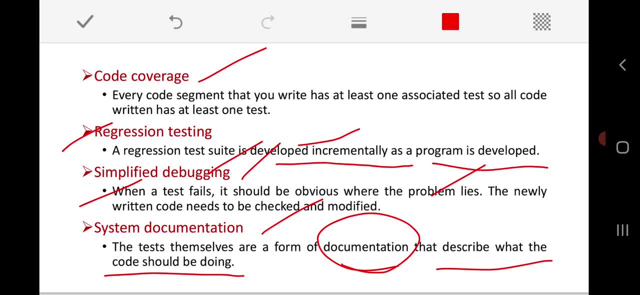 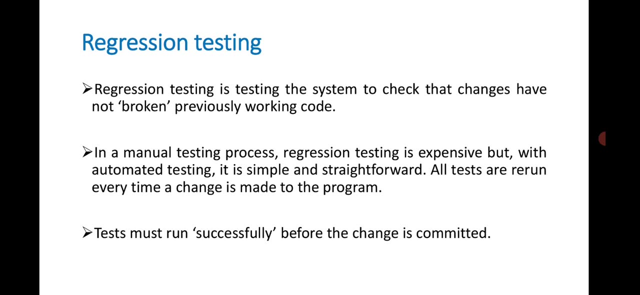 stand in future, okay, with all these different sort of testing that we might have done on a series of our implementation of what the coding is concerned. so these are the different benefits and just now, as i told that, in case of regression testing is concerned, okay, this regression testing is.